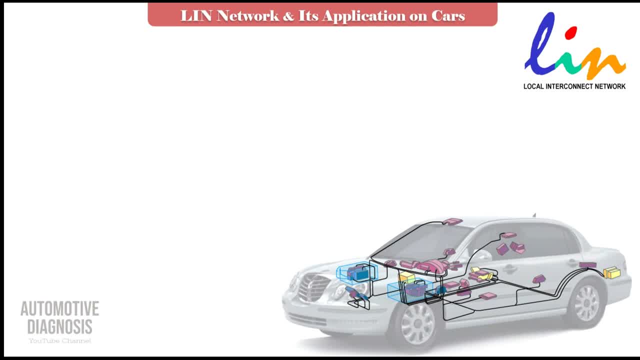 couple of other videos about the network, mostly on CAN bus, and after publishing those videos I received many messages and comments to make a video about the Lean Network as well. so that's why today I'm making this video for you guys. First of all, we will start by having a look at the Lean Network Basic. Normally, when we are 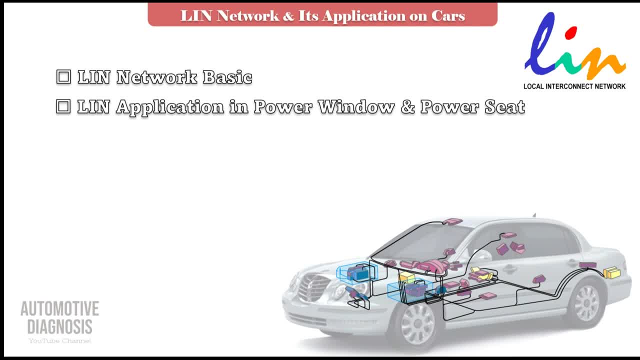 talking about the Lean Network. you guys are supposed to know where to find it, So I'm going to show you some really good examples about the Lean Network on the wine diagram and a couple of experiences as well. So you, you, you will- at the end of this video, you will know the application of the Lean Network. Then, after having 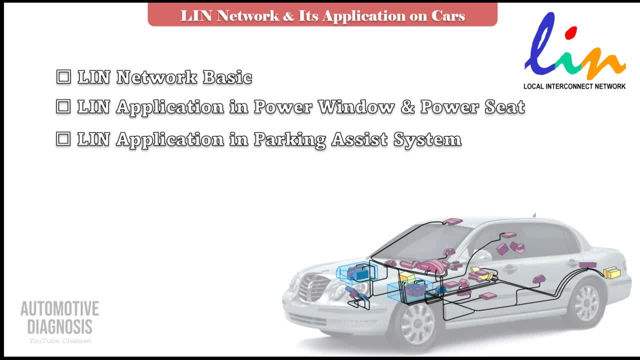 a look at the power window and power seat application. we will continue by having a look at the parking assist system to see how Lean Network is used in parking as a system. Then we will have wiper and the rain sensor, because Lean has been used on wiper and rain sensor as well. 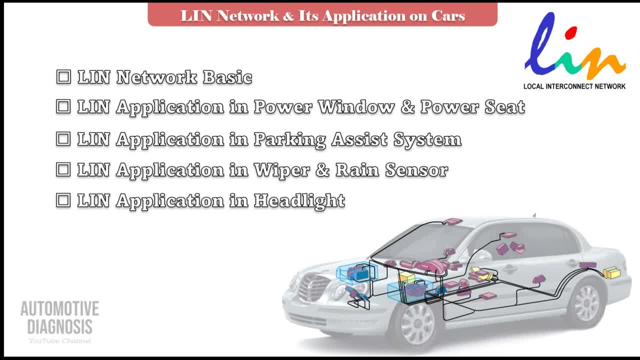 Then it's going to be the headlight. So we we are going to focus on the main subjects and main systems and it doesn't mean that you you will not find Lean Network in other systems as well, But these are the major and main components using Lean Network and if you watch this video and if 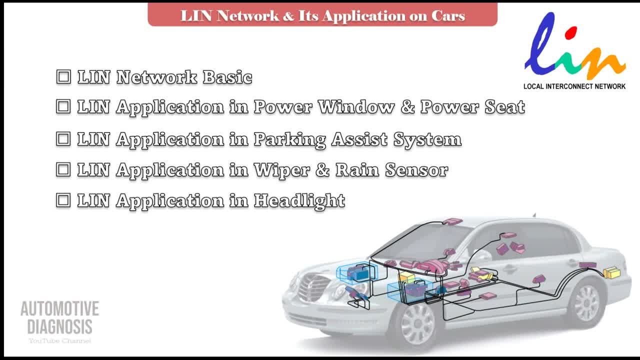 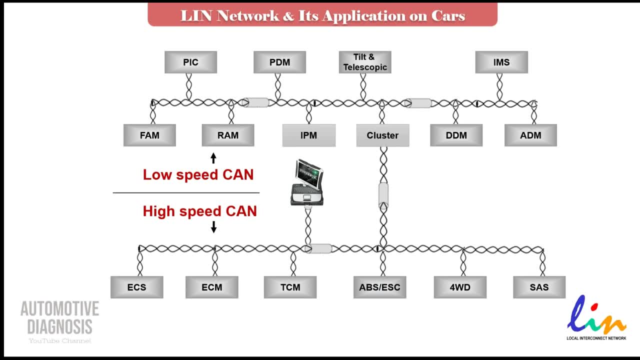 you know how lean works. obviously it's going to be super easy to find the Lean Network in the other systems, just by having you look at the wiring diagram. All right, so, as I said earlier, we have a couple of other videos for the CAN bus. I will leave the 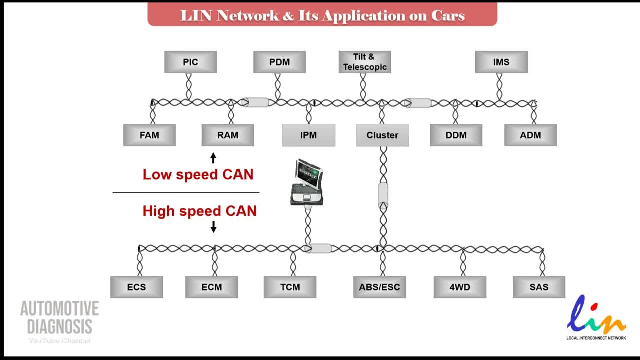 link of those videos in the description so you can watch the CAN bus structure and Diagnostics video as well. But basically, when we have the network in the car, I'm just giving you really, really quick idea about the network, Then we will see. why do we need to have a lean network? So basically, network is designed to 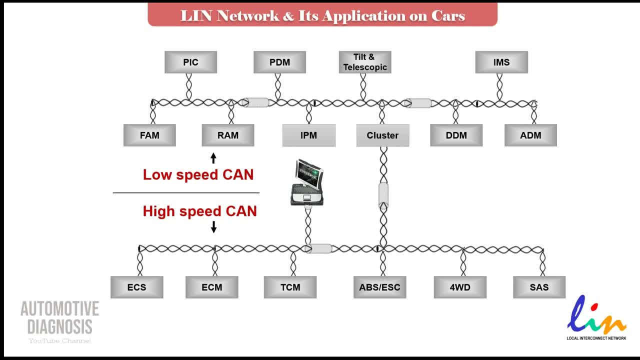 minimize the need for having the wiring because you see all these control units, you may have even more than these control units on one car. So it means when you have so many control units and when they are communicating to each other, you need to have so many wires and wiring harnesses in the car. 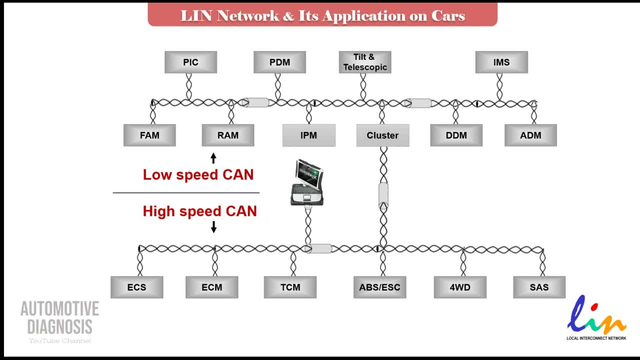 And I'm not really worried about the cost side. I'm just worried about the diagnostic side. When you have so many wiring, it means you may have so many problems, Connectors or the wirings. they are normally the source of the problems. So companies are using the network. 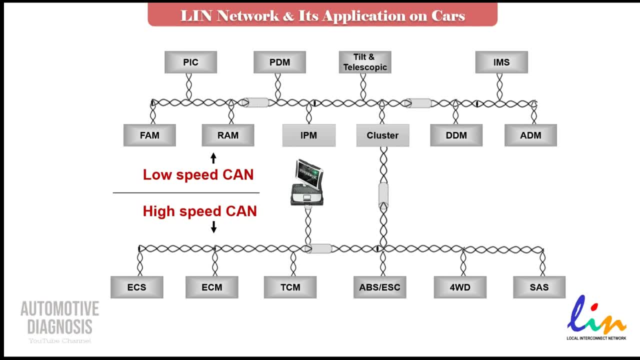 to minimize the wiring and the wiring harnesses. This is the first one And, on the other hand, 3 using the network is going to give this ability to the power is to share the information between the control units at higher speeds. right, because when you are 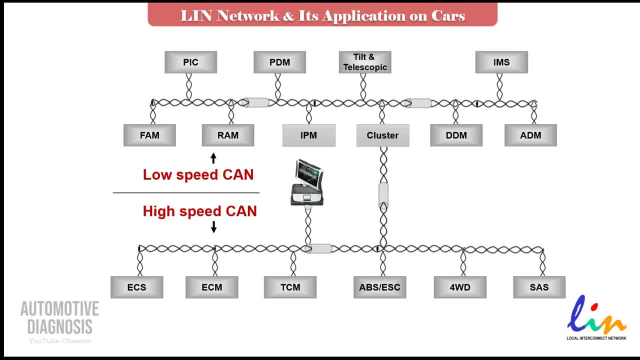 using a normal hard wire. so control units are sending the signals as usual, just the voltage or whatever they are sharing to each other. but now, when they are using the network, information will be shared at really high speed, for example here on high speed. can all these control units 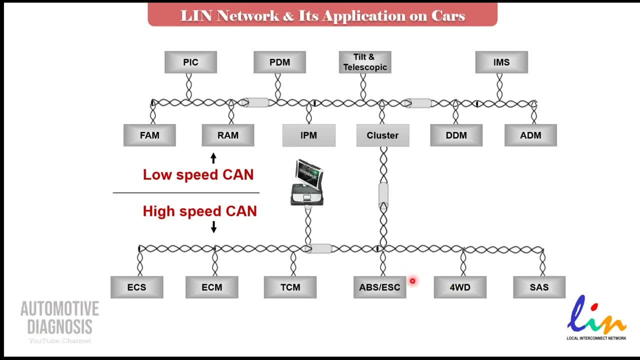 are connected to high speed can, so they will share the information using this network and the speed that we are using in the high speed can can reach to one megabit per second. so it's going to be very hard- higher than the normal hard wiring and on the lowest bit can that normally we call it. 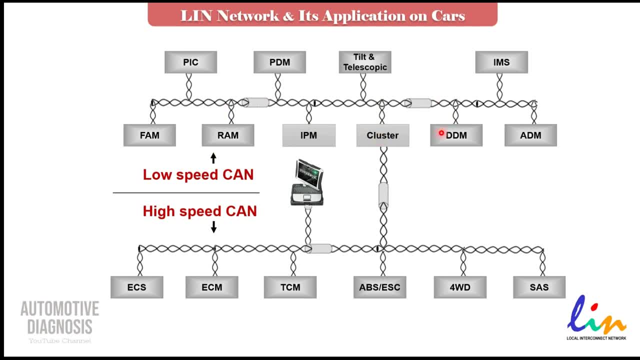 body. can you see some other control units like the driver door module, assistor module, power seat and a couple of other things? uh, other control units. they are sharing the information at lower speed but still it's, uh, it's not comparable to a normal hardware, because in low speed can we can reach up to 125 kilobit. 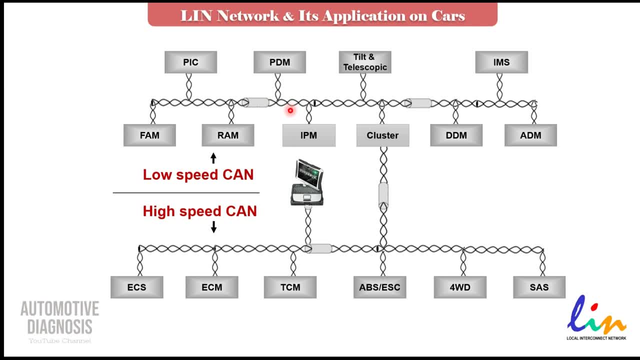 per second, which is still really good speed. so when you see these two uh classes of can right now, you see those control units which are really critical, like engine uh brake system transmission. so these are really sensitive, really critical. we need to send the information and we need to share the information between these control units as quickly as possible. 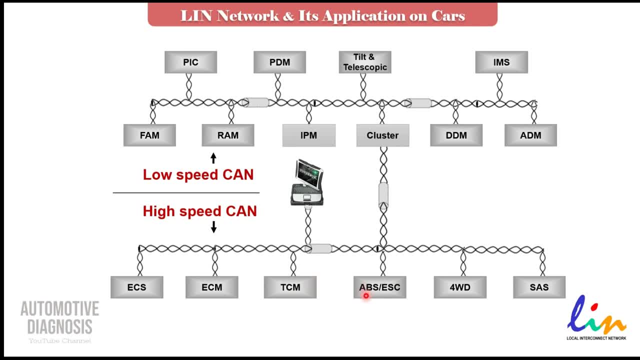 that's why we are using the high speed can. but the other control units right here in the body can? they are less critical, all right, so it doesn't mean that they, their information, is not important at all. of course it is, but this information is not as critical as 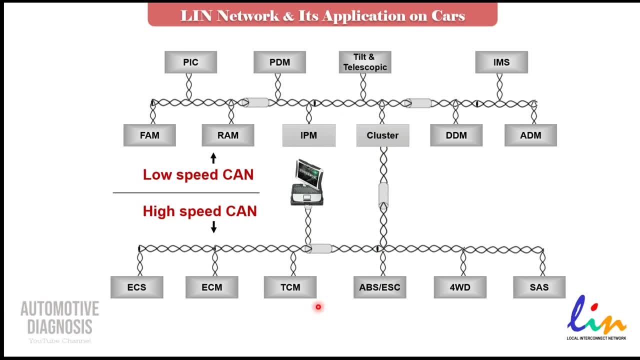 uh, these information in the units in high speed can. so that's why we, when we are using the lowest speed can, we are still using the network, but we will have less speed compared to the highest with here. so, uh, when obviously you are using less speed, the total cost of creating these control units? 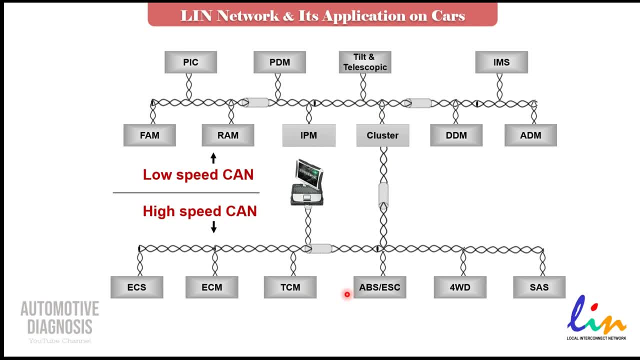 is going to be less than the high speed one, but is there any need for sharing other information? yes, of course. of course there is. so we already know about the lowest speed can and high speed, but sometimes there are some other components, mostly some sensors. they need to communicate, uh, with these control units connected to the beacon or to the 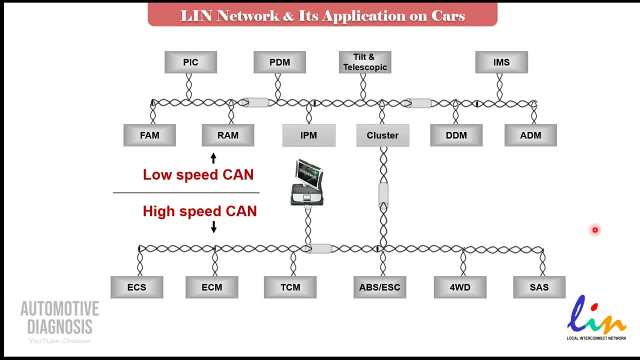 highest speed cam right. so it means, if we have other components which are even less critical than these, control units in the lowest speed can, instead of using this kind of network, instead of using the can network, we're going to move to another network, which we call it lean network. so in the canvas, if you watch the other video, 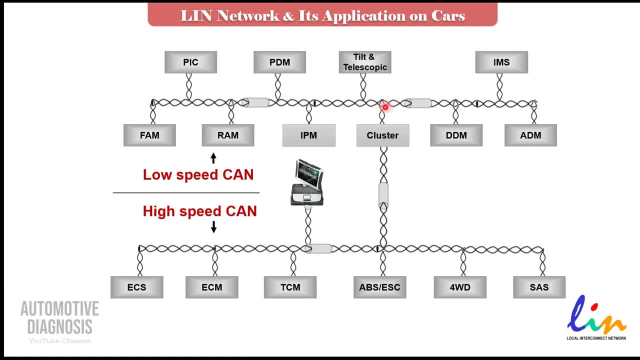 in the description you see that the canvas is using a pair of twisted wires. so it means you have two wires which are twisted to each other in the can network and the speed that you reach is one megabit per second in high speed can and 125. 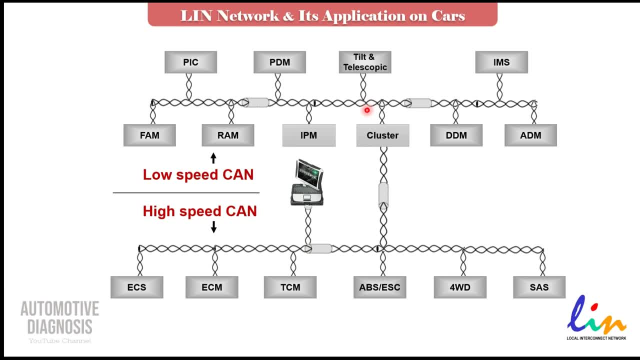 per second in low speed can, but if you have any other component, uh which needs to send the information, which needs to share the information- less critical as low speed can, but still you are trying to share the information, uh, faster than the normal hard wire- we can move on to another. 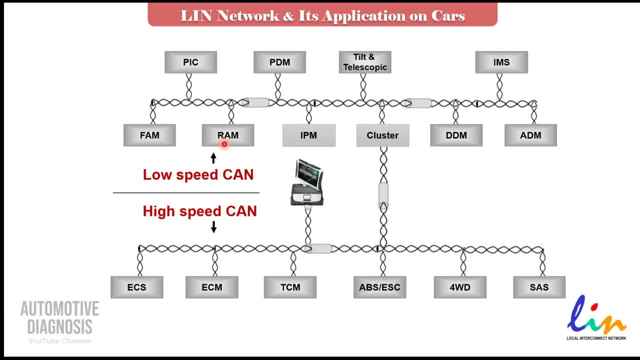 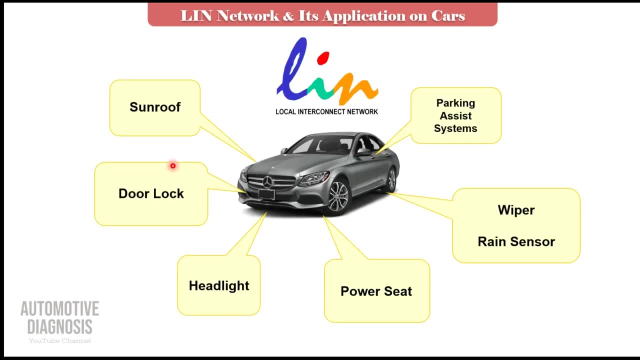 network which is less critical and which is going to cost way less than low speed cam. so that's the first one that you'll notice here. the most important one is lean network. so lean is the abbreviation of local interconnect network, local interconnect network and in the lane network we 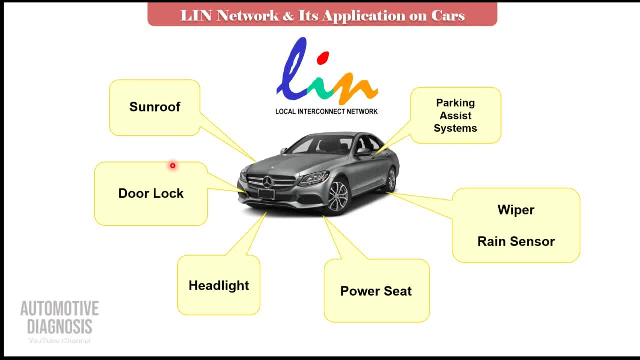 are using only one wire- only one wire, not two wires anymore. like the can network, there is just one wire to communicate. so normally you can find the lean network in these systems, and obviously So. I've seen the lean network in sunroof, in the power door lock system, in headlight that we will see today- in power seats, in the wiper and rain sensor and sometimes in parking assist systems. 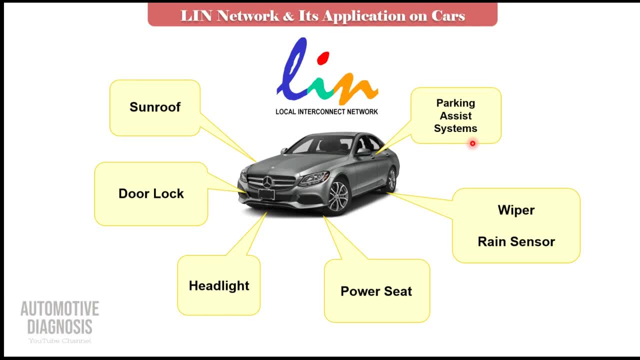 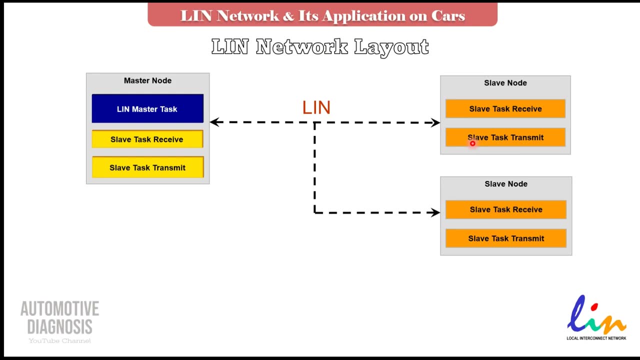 And obviously, as I said earlier, in some other systems as well. So let's have a look at the structure of the lean network. Then we will start talking about the different systems using the lean network. So this is a simplified structure of the lean network. 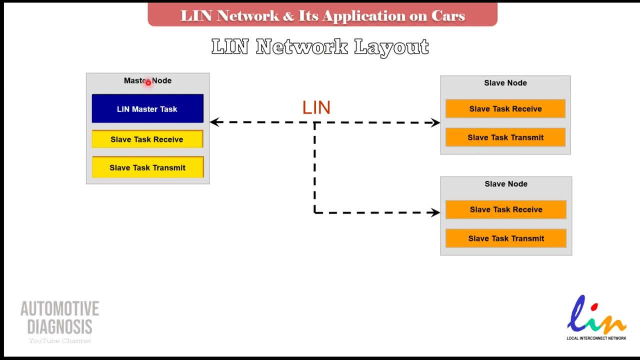 So normally on the lean network we have one master node, which is normally your control unit, and there are some slave nodes, So these are normally your sensors And, as you see, there is only one wire which is lean network. So this wire between the master node, between the master node from here to this slave and the other one, 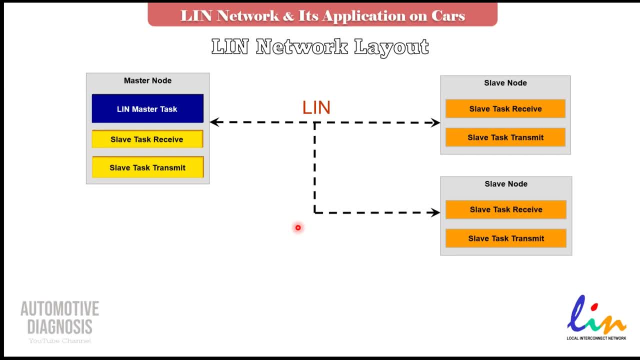 And then you have the control unit. The important point is, you don't need to separate lean line for each node, all right, So the master node is sharing only one line, all right. And, as you see, these two are connected to each other. 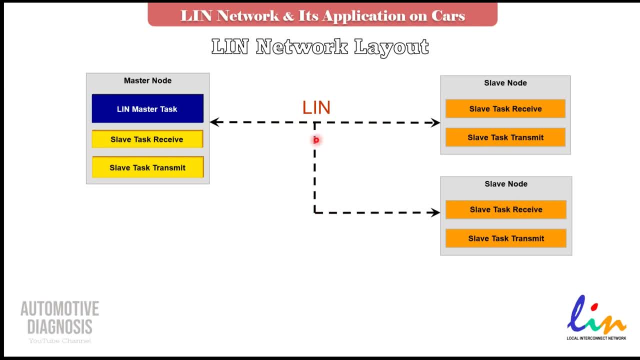 So this is going to minimize the need for wiring even more. all right, So this master node is going to be your control unit. The slave node is going to be your sensor which is working on the master node. If you remember, the CAN bus- CAN bus is some sort of multi-master network. 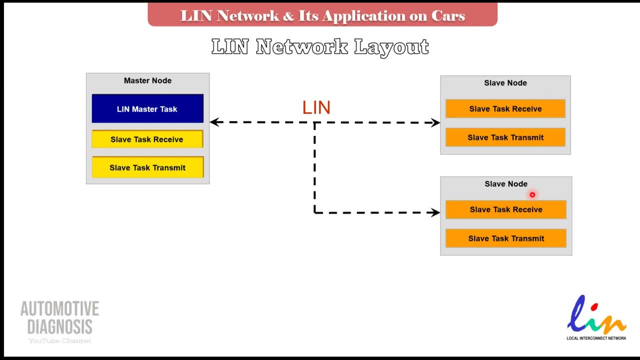 So all the units connected to the CAN network. they are a master node So they can share the information and receive the information or request the information from the other control units. But on the lean network we only have one master and multiple slave. 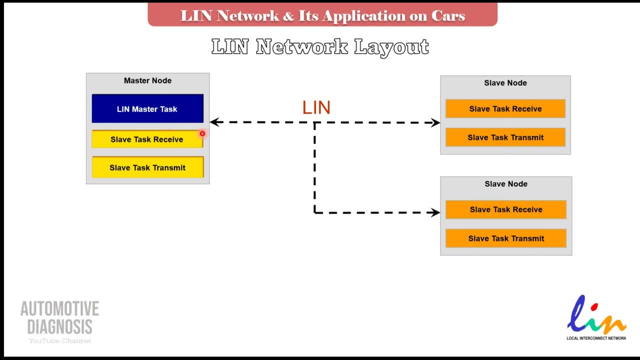 Okay, one master node and multiple slave nodes, So this is going to minimize the need for wiring even more. So, for example, if you are talking about the parking as a system, master node is going to be your control unit and the slave node is going to be all the parking sensors. 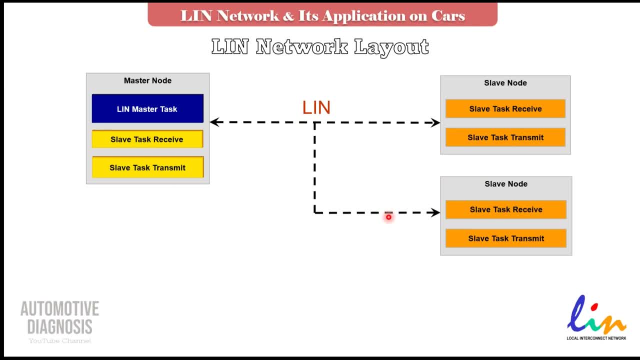 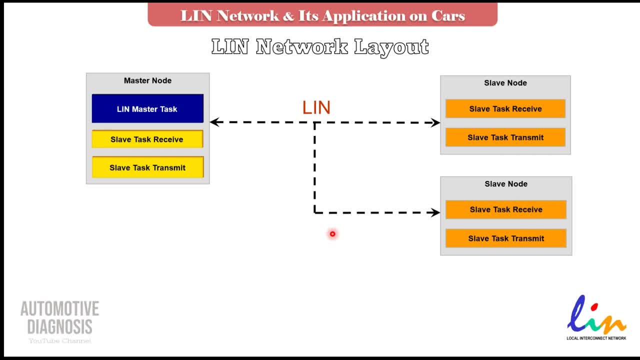 So this is going to minimize the need for wiring even more: Kilobit per second for the low speed CAN and one megabit per second on the high speed CAN. So this one obviously is way slower than the other kind of networks, but still much better than the normal hard wire. 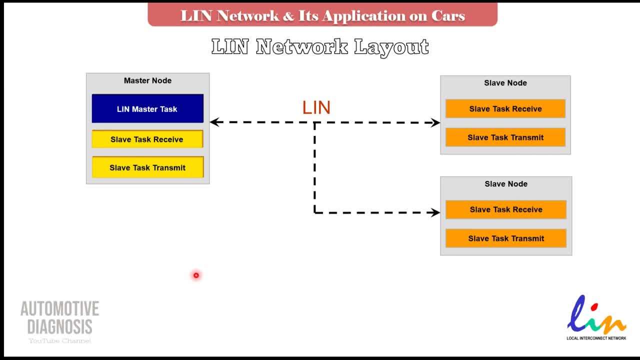 And normally the voltage in the lean network is going to be 12 volts, is using the 12 volts And normally this is what we get if you check the waveform on the lean network. All right, Let's start to have a look at some systems using the lean network. 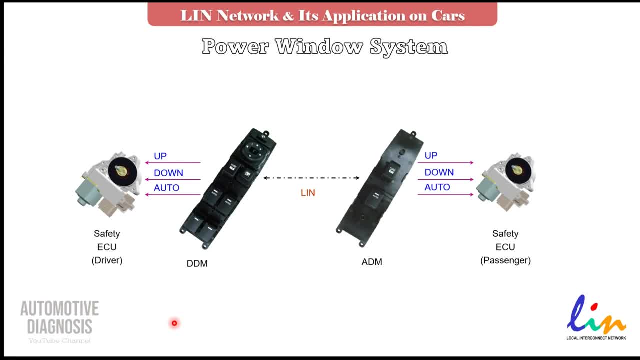 So you guys will know how to find it in the wiring diagram. So on some cars the communication between the driver door module and assist door module is via CAN bus- low speed CAN bus. But on some other cars this communication is going to happen via lean network. 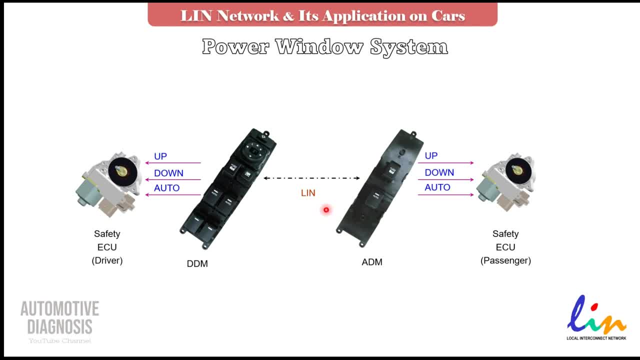 Right, Because this communication is not really critical And they can reduce the cost by using the lean network instead of the body CAN. So what happens? For example, you have the power window If you are trying to open or close the other window. 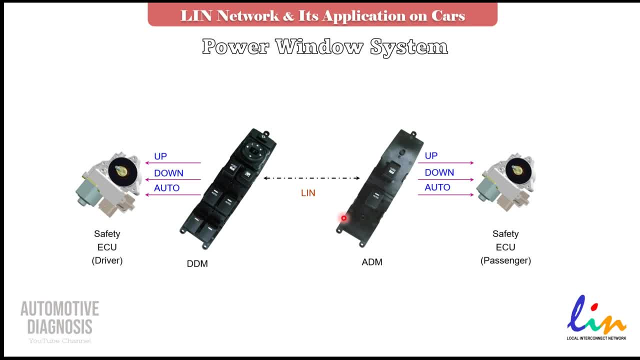 Or, for example, you're sitting on the driver's side. You are trying to open and close the driver's side, then necessarily, uniqueness- well, you're on your driver's side. or close the power window on the passenger side. normally when you are. 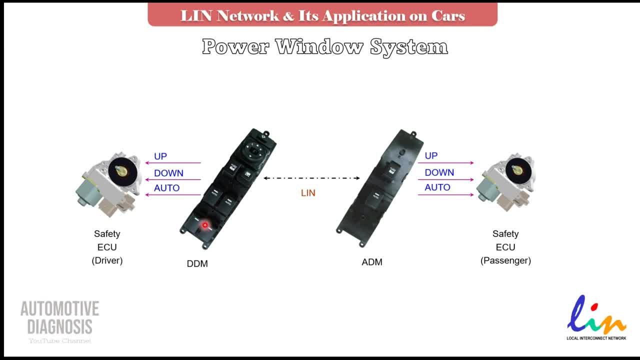 requesting from here, when you are trying to open or close a window from here you are communicating to as a store module or passenger side door module, we are lean network, right? so it means, if we didn't have lean network, what was the situation? so you needed one line for the closing request when you wanted to move. 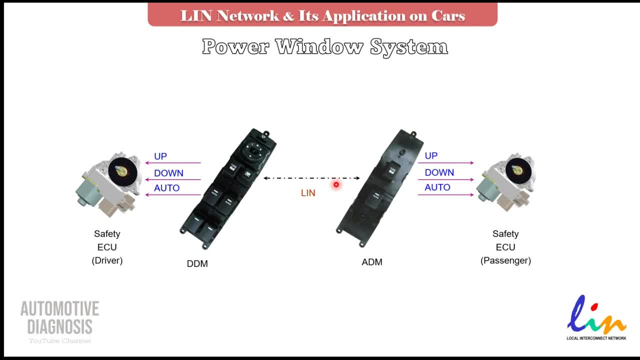 the window up and for the down right, for different requests, you needed one individual wire, right. but right now you are just using one wire, which is your network. so right now your door module, so right now your driver door module is communicating to as a store module. we are lean network and really doesn't. 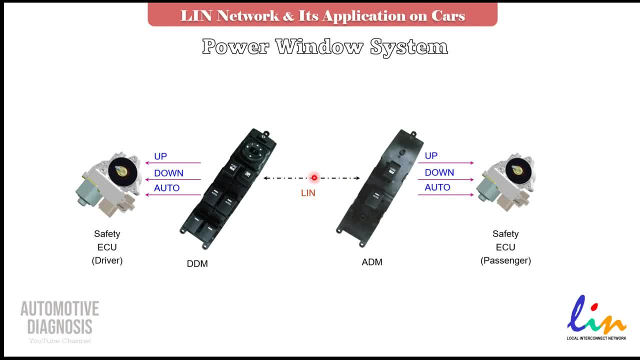 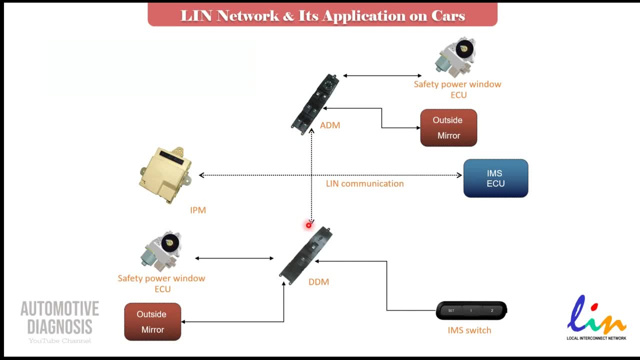 matter how many different signals they need to share with each other. they're going to use just only one wire, which is the lean network driver door module and, as a store module, are using the lean network and IMS ECU is exactly the power seat control module with with the memory. 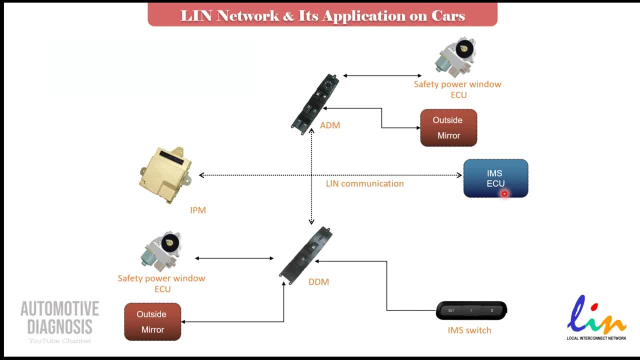 okay when you can memorize the situation of the power seat. so, as you see, the power set control module is communicating to IPM, which is which is your fuse box, will be a lean network as well. so in normal situations, these four control units needed to share so many. 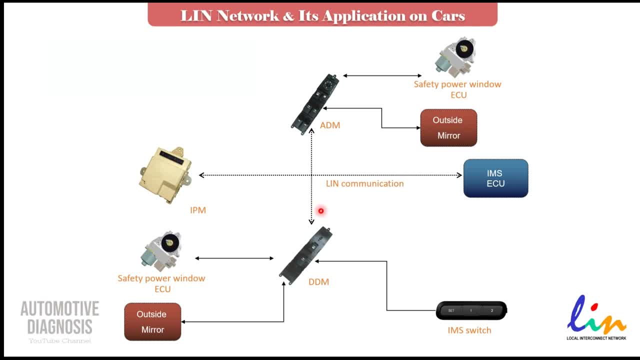 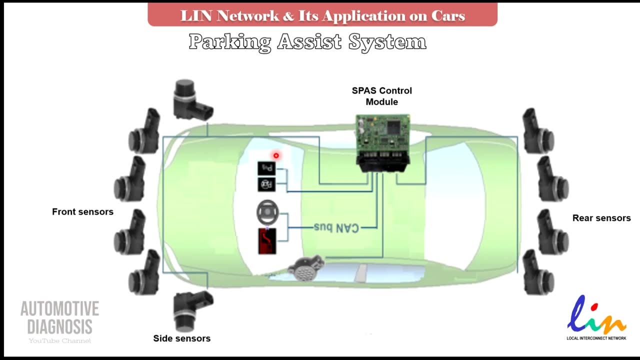 wires, but now they are just using a normal lean network. all right, guys. next one is parking as a system. so, as you see, on this parking as a system, we have the smart parking as a system control module right here for sensors on the real sites sensor on the front side, and we have two side sensors. we may have two other side. 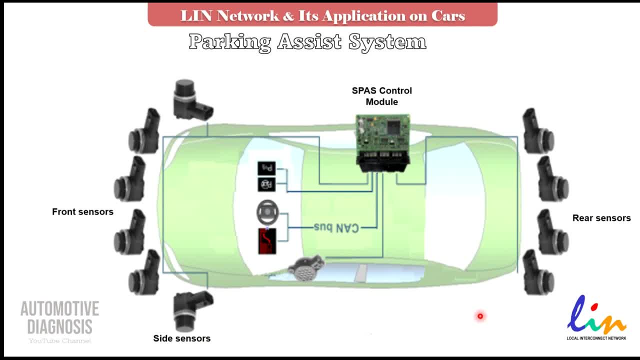 sensors in the rear side as well, based on your car and, as you see, all these sensors normally need to communicate directly to a smart parking as a system to send the information, to, say, can send a signal, but right now they are using just a lean network and the information is shared at high speed compared to the 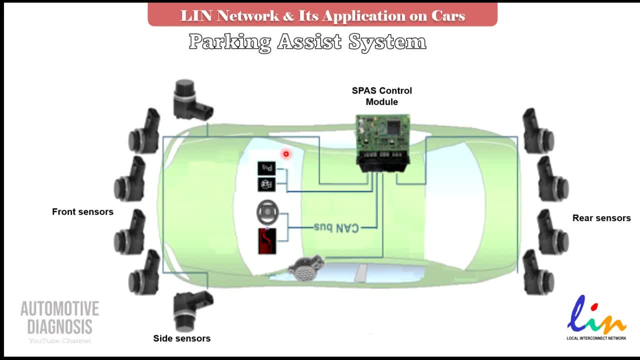 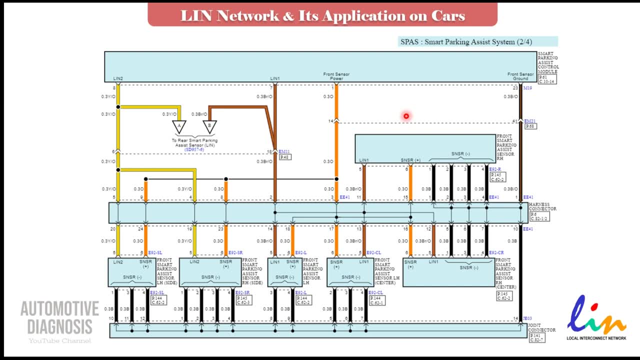 normal wire. but let's see how this lean network works on the real wiring diagram like this one. so this is the wiring diagram for smart parking as a system and, as you see, this is the control module up here and right here we have two lean networks: lean 1 and lean 2. so if you focus on lean 2, lean 2 goes. 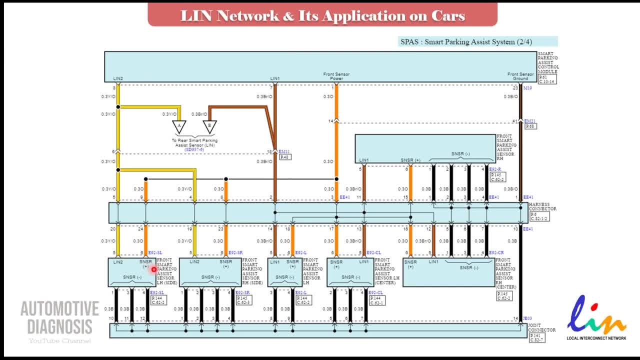 all the way to side sensors. so this is the side sensors. as you see, this one is side sensor, the other one is side sensor as well, right, so these two side sensors are connected to lean 2 and lean 1. with this color, this one is connected to all front parking assist sensors. right, but they. 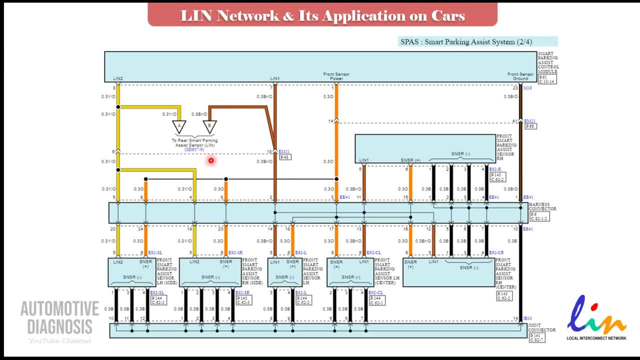 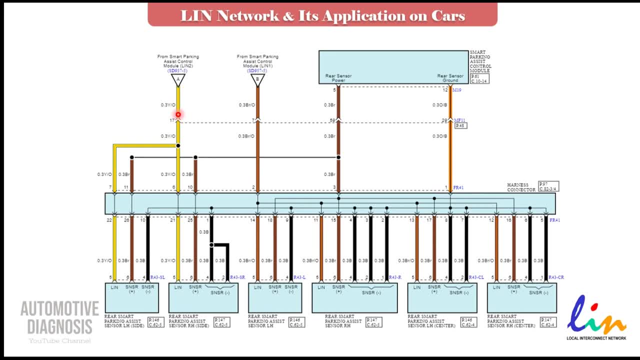 are going to the rear parking assist sensors as well. on the second page we have again lean 2. we have again lean 2 for another two side sensors on the rear side, because for this one we have another two side sensors on the rear side and lean. 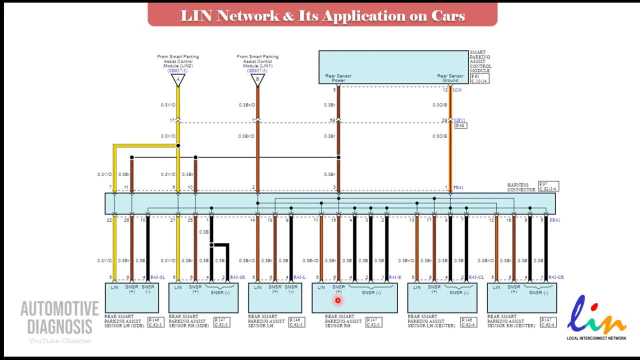 1 again is connected to four parking assist sensors at the rear side. so it means lean 1 is connected to eight sensors and link two is connected to four sensors. so this is how you can find the lean network on the wine diagram and, as you see, I just like a normal wire on the. 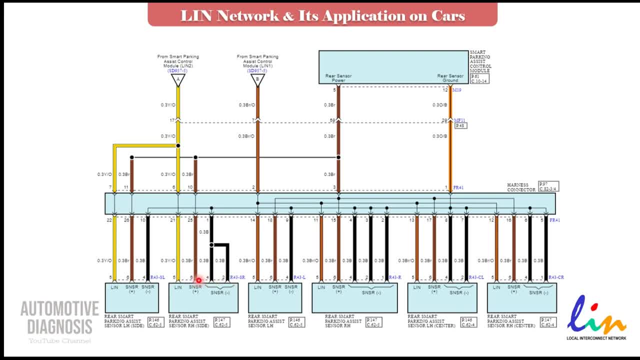 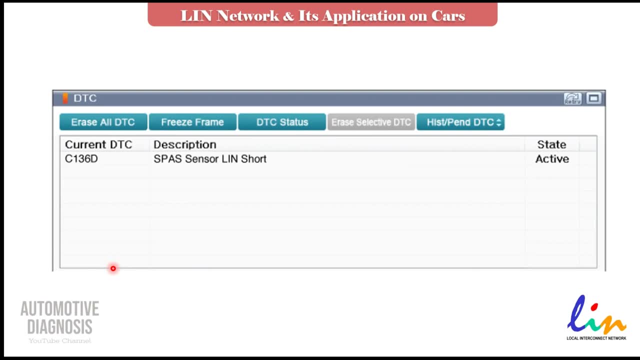 sensor. so right here on the sensor you have these pin numbers two, four, six and five. number five with this wire color yellow and orange. this one is the lean network and same on the other side as well. so what will happen if you have any fault on the lean network? I'm going to show you one example from actually what 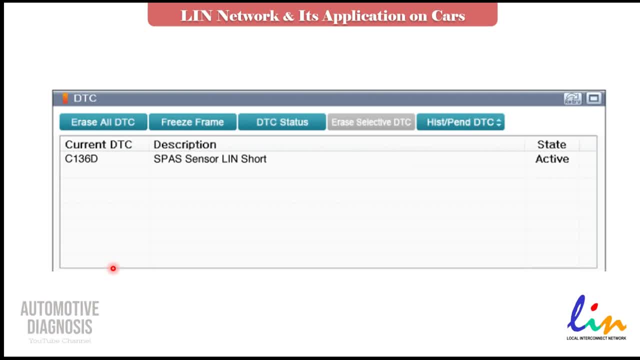 I had one time on one car I had. I had a Kia Sorento 2017 one time and the problem was car. that car had a crash from the rear side, from the rear left, and apparently customer took the car to a panel beater. they just replaced the rear bumper and 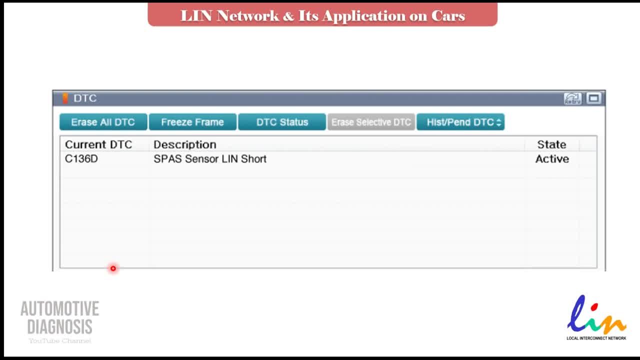 apparently they tried to remove and put remove the sensors and put them back on. but right after finishing everything, after finishing the panel beating job customers, saw a fault on instrument cluster for parking, for a smart parking system. and when he brought the car to our workshop, when I checked the car, I 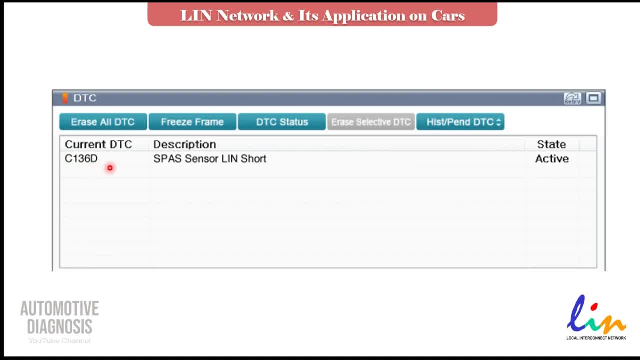 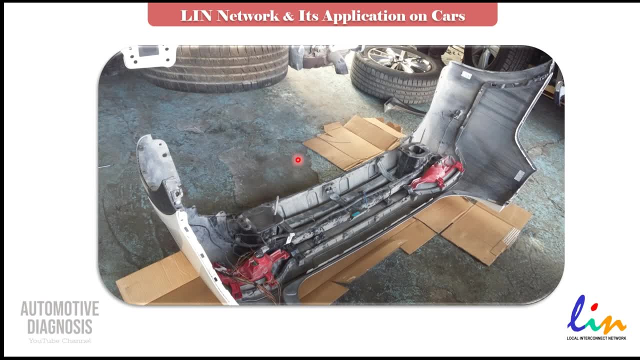 had this fault- uh, C136D smart parking assist sensor, lane shorts. and when I removed the rear bumper- this is the bumper when I removed it, you see this bunch of wiring right here- I removed the bumper and I- because I was just trying to see what's going on with the sensors- 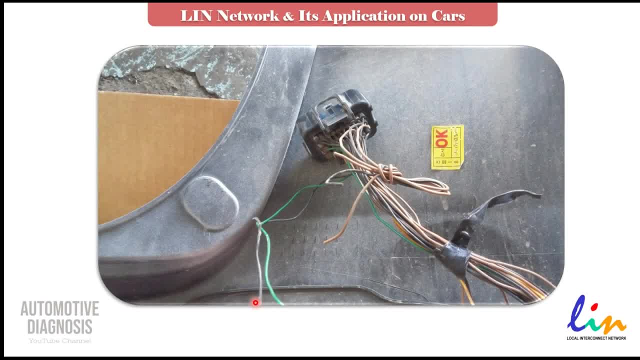 I removed the whole bumper and this is what I found. you see these wires, this one and this one. so apparently this guy who was doing the panel beating job or the one who replaced the rear bumper, they didn't know how to fix the problem. on a smart parking assistant system, they just cut the connector from. 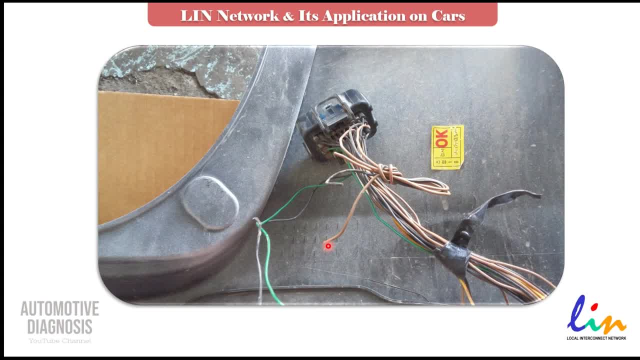 one sensor and this is what you see, because maybe the connector was broken after the accident or whatever, because I couldn't find the connector anyway, they just cut this wire, and one of them is the lean Network. uh, because I wanted to see if the problem is just right here. 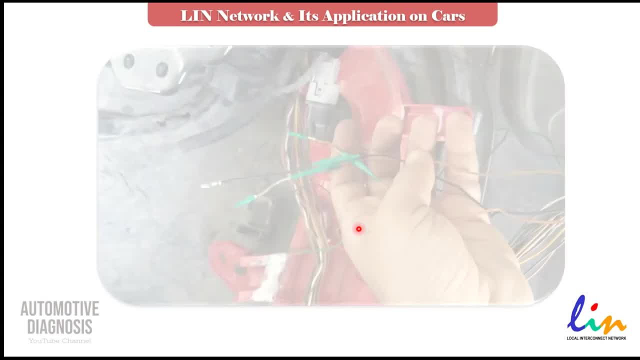 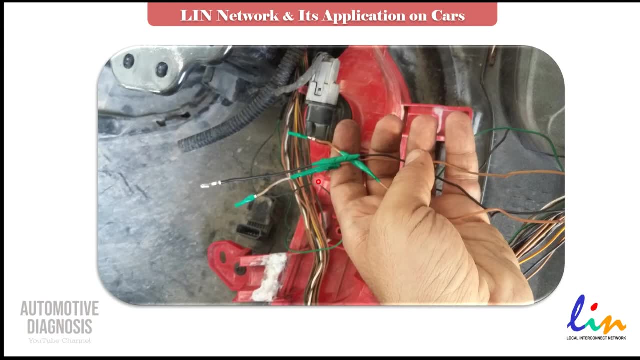 or in any other place in the wiring. I just try to uh fix the wiring uh just quickly, just like this: I put some pins on the wire, on the on the wires, okay, to secure them uh inside the sensor to see if the uh fault code is going to go away. so, after uh crimping these pins on the wires and inserting 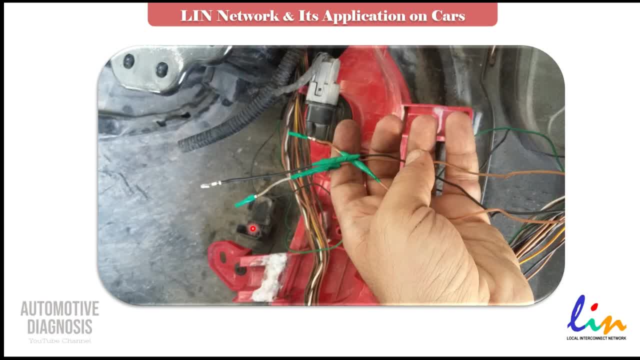 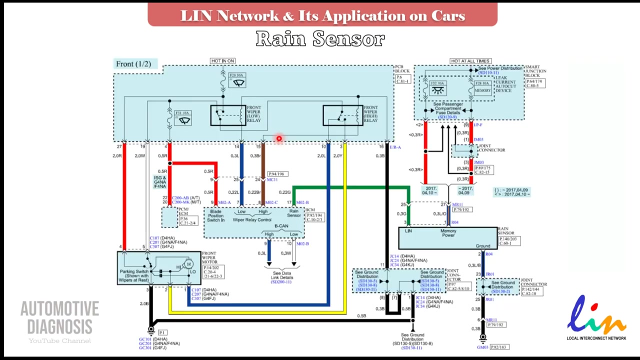 inserting them to ins into the sensor, everything, uh, everything started to work as normal and we didn't have the fault code anymore because, obviously, technically, they did, uh, they cut the wire and this cutting the wiring caused some short circuit as well. so, uh, we had this. we had this problem on the lean Network. so the next: 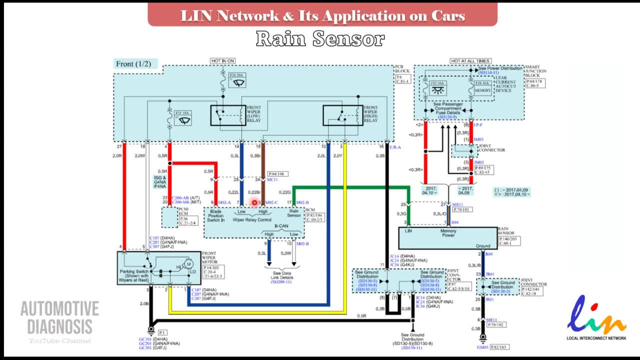 one is the rain sensor. as you see, this is the wiper system. we have the body control module here, uh front wiper low speed relay and the high speed relay. so obviously body control module is responsible to energize the relays based on uh customer request. but when you have the rain sensor, 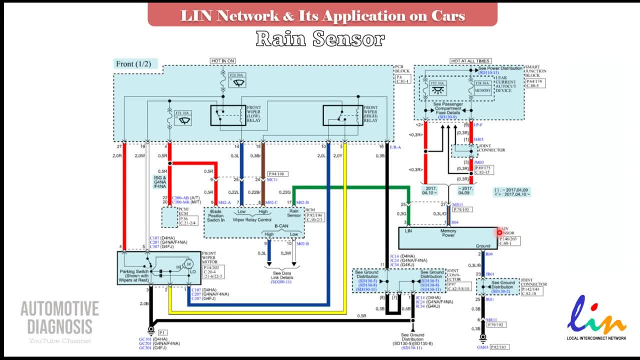 it means anytime that you put the uh wiper switch on auto mode. what happens if? if you're driving and starts raining, rain says a drain sensor is going to detect that and it will send the information right to energize the wiper relays. but in this case, as you see, we have only lean Network, we have only 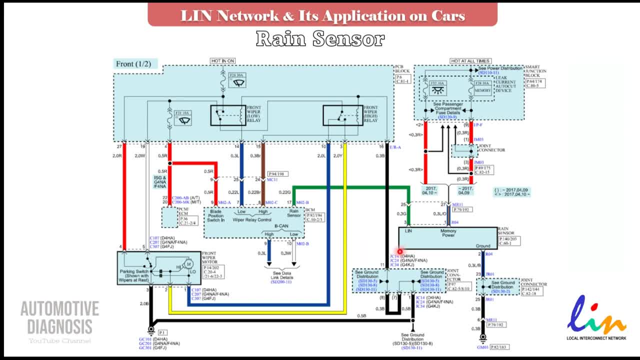 lean Network. instead of having a couple of wires for communication between rain sensor and body control module, we only have one wire, which is the lean Network uh between the BCM and between the rain sensor. so anytime that uh that is raining after rain sensor detects that it's going to share. 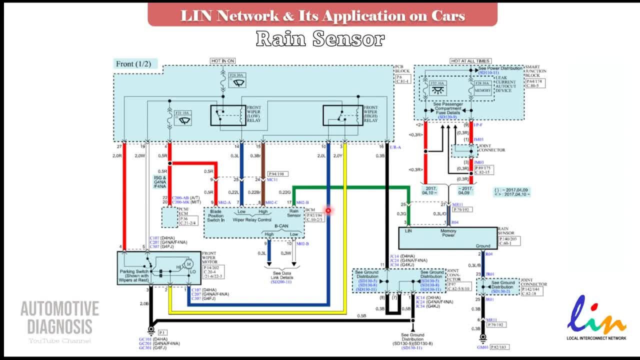 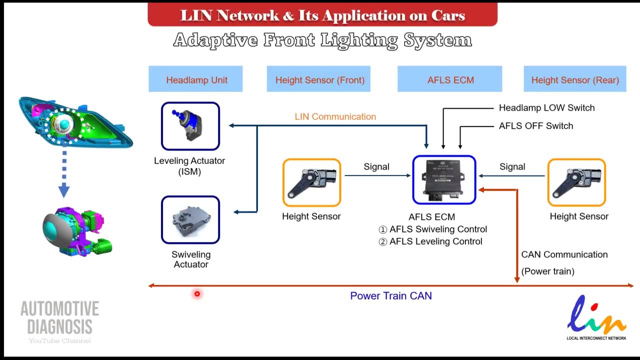 the information uh to the BCM. we or YODC, this uh lean Network, and BCM is going to energize the wiper relay to operate the front wiper and the last one for this video is adaptive front lighting system or AFLS. so on this system as well, as you see, we have some actuators uh in front. 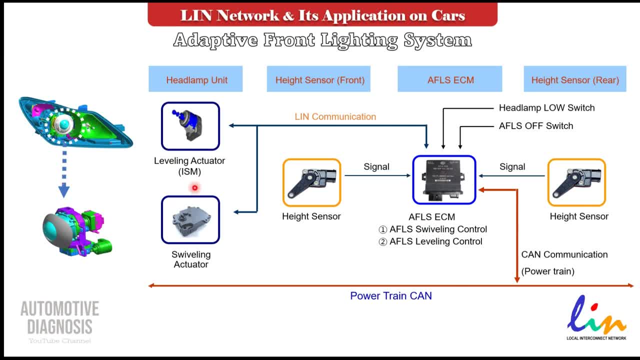 lighting system: uh for, uh for leveling, uh the headlights or uh to adjusting the headlights when you're cornering. so for this one you have one control unit, uh, some sensors to detect the vehicle height and the actuator. so in this system, control module is communicating with actuators. 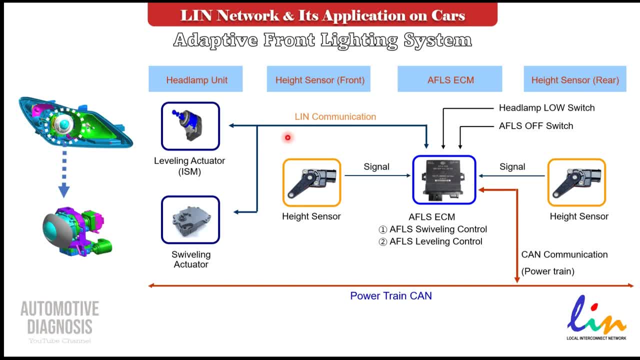 using the lean Network. so so far we had the sensors. now we have the actuators. so for different mode of actuation- because the leveling actuator has different mode, and even on the cornering. so instead of using all those wires for actuating the actuators in front lighting system, we only have one in Network and 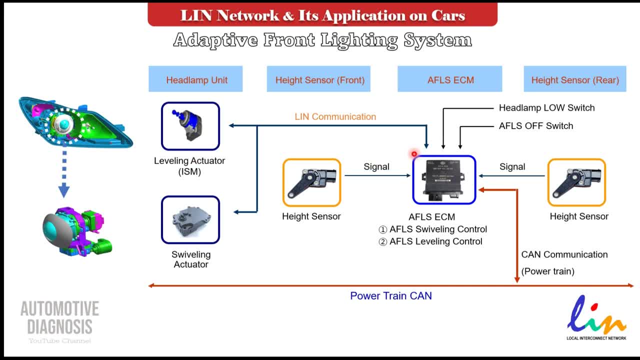 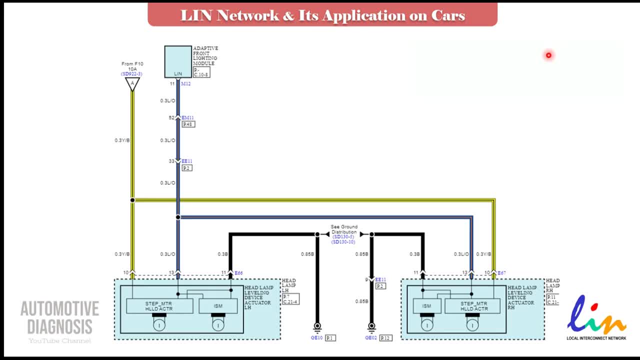 as you see, even these two actuators are using very same uh lean Network. okay, let's have a look at the wind diagram for adaptive front lighting system and, as you see, we have the control module and we have the headlights- uh, left side and right side in here. 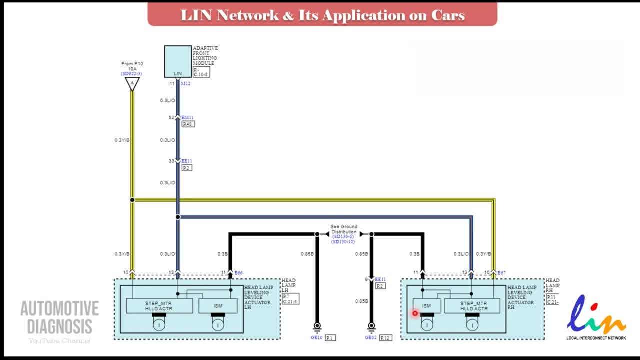 and, as you see, we have two actuators, two actuators in here. so, uh, so all the control functions for these actuators are controlled just using one lean Network. so it's one lean Network connected, the control module, and it's shared between the left side and right side. 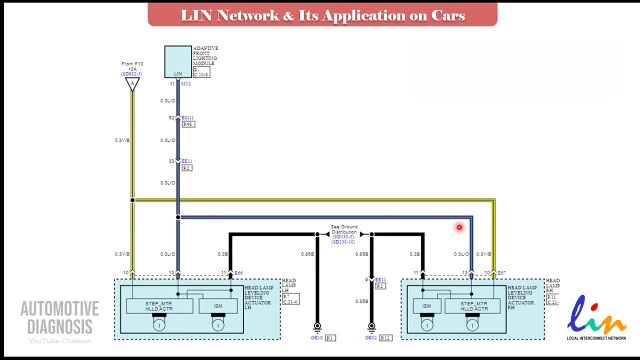 uh headlights. so instead of using uh so many wiring, we just have one in Network, which is quite reasonable. so this is a code that some- sometimes I, I- had for the lean error on adaptive front lighting system. normally when there is a short to battery or short to ground in the lean Network and surprisingly, a 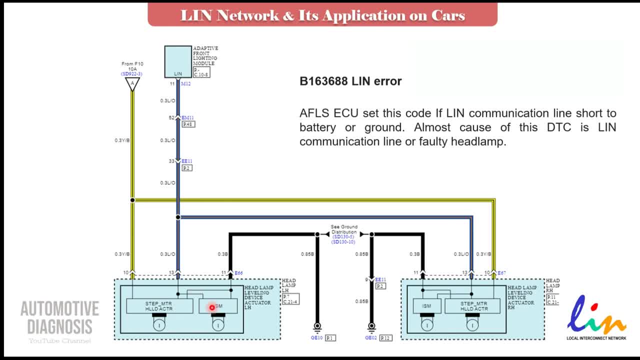 couple of times I had this fault because of the internal short uh inside the headlights. so the light was okay, the lean Network itself was okay, but after headlights replacement everything was back to uh, everything was back to normal. so you need to keep it in your mind that sometimes 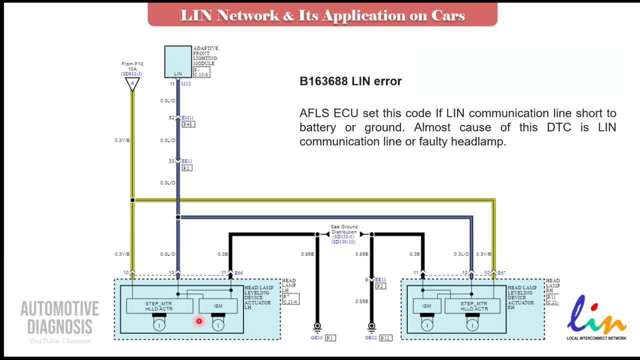 I like light can. uh, we may have this fault on the can as well. internal problem or internal short inside the control module on the canvas receiver. we may have this fault on the lane Network as well if there is any short, any internal short in in the slave node. 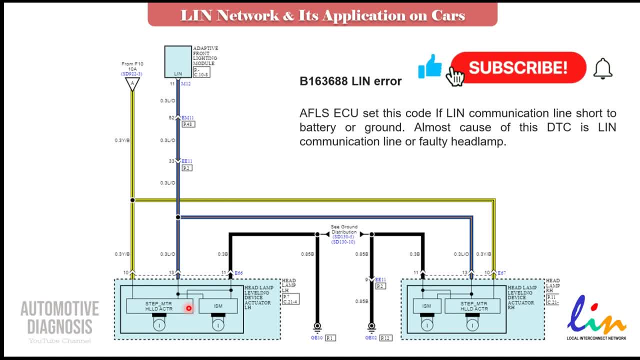 All right. thank you very much everyone for watching this video. Please don't forget to have a look at the other video for CANBOSS network if you haven't watched it so far, And if you like this video, please don't forget to like it. 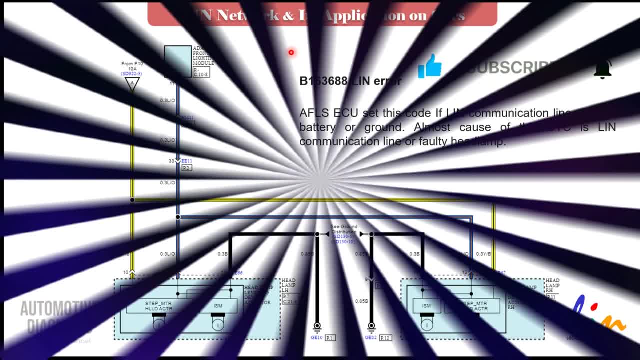 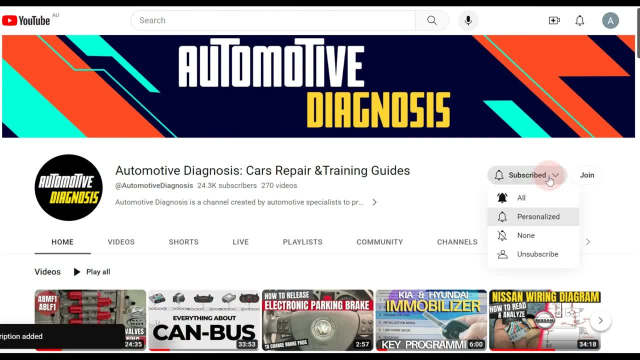 and share it with your friends. Subtitles by the Amaraorg community.